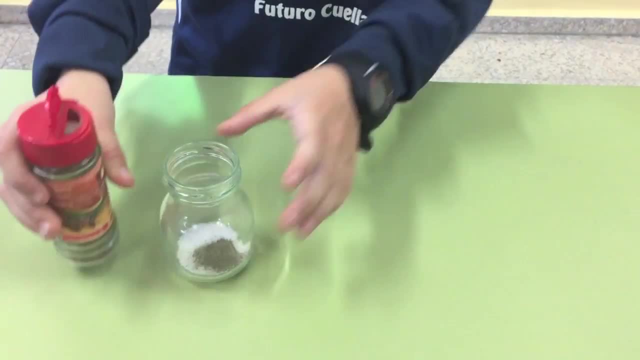 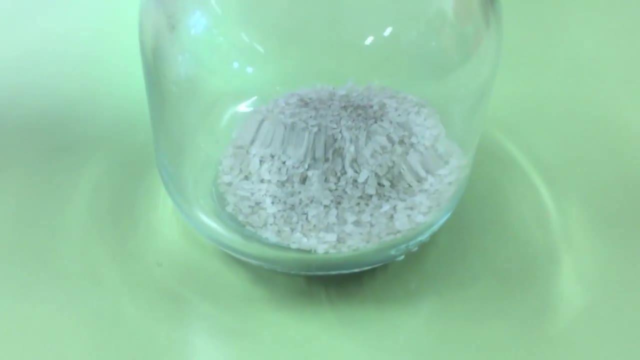 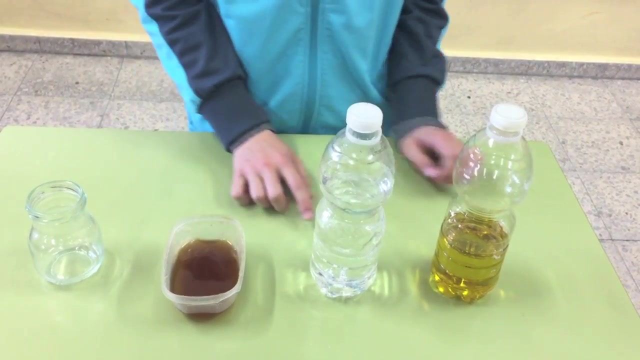 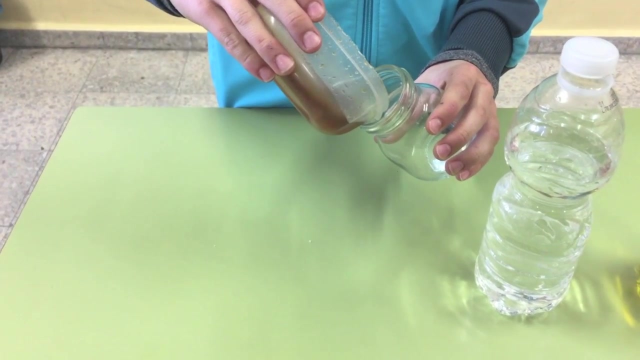 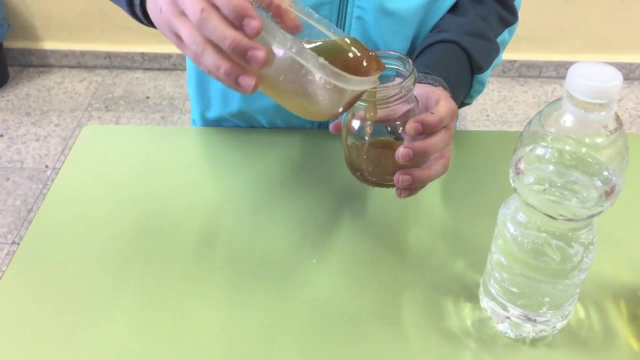 put the pepper with the salt and we mix. we can see all the components, the salt and the pepper. This is another example of heterogeneous mixtures. We mix honey with water and soy. First, we mix the oil, Second, we mix with the water. 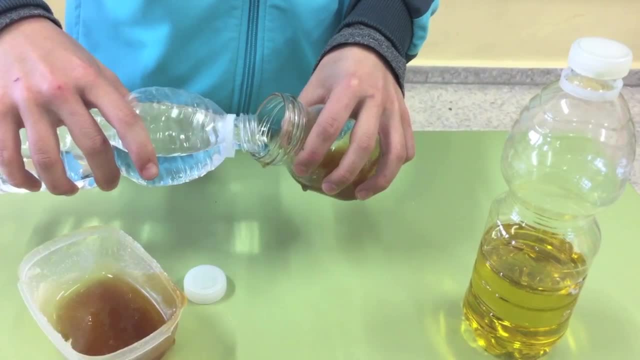 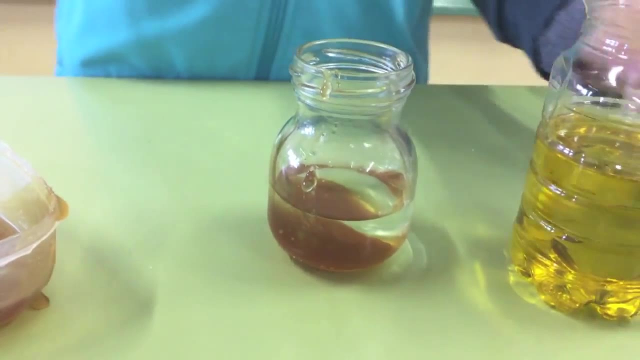 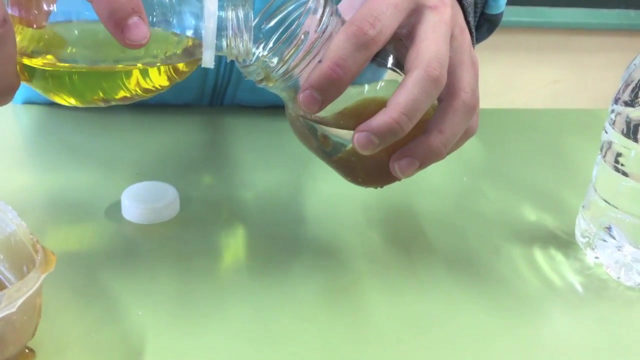 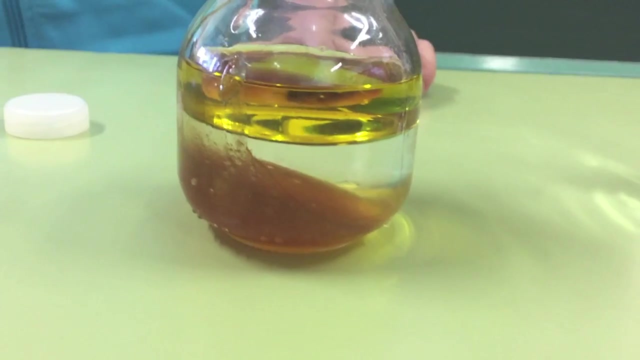 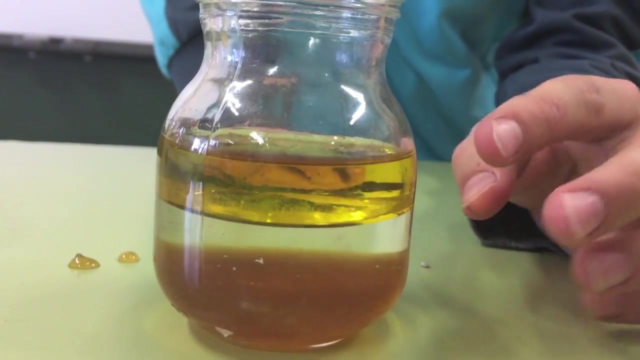 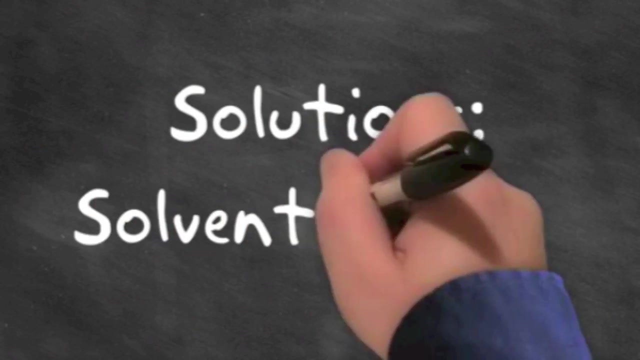 And third, we mix with the oil. And third, we mix with the oil. And third, we mix with the oil. You can distinguish that in the upper part is the oil, that in the middle part is the water and in the lower part is the honey. 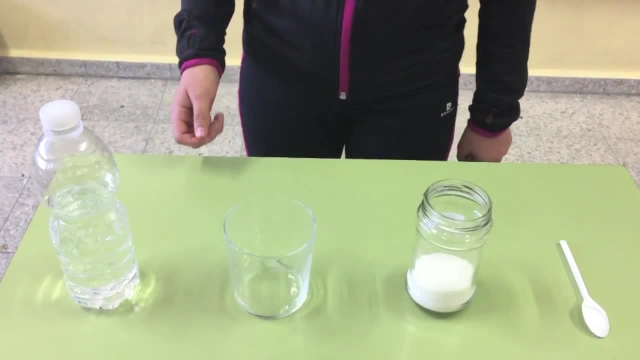 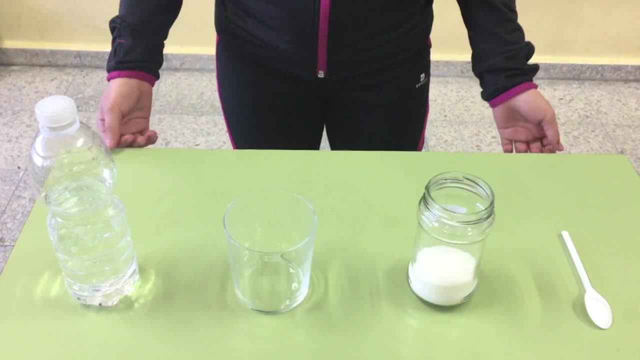 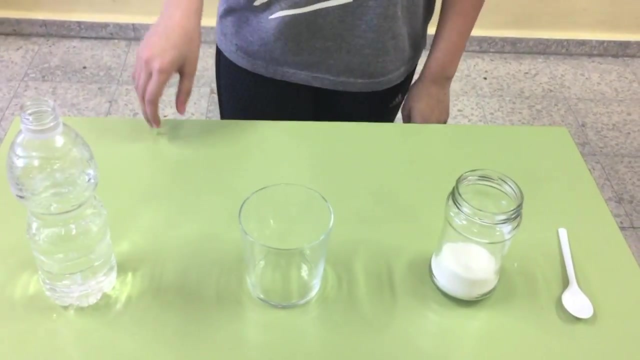 We are going to do a solution that is a mixture of a solvent that is a liquid. in this examples is the water. can be a gas or a solid that, in this case, is sugar. For doing this experiment, we need to put some water. 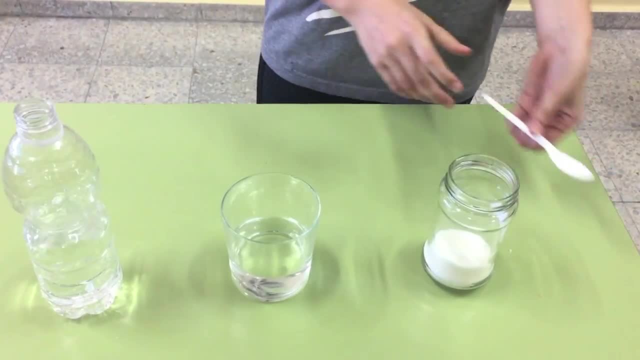 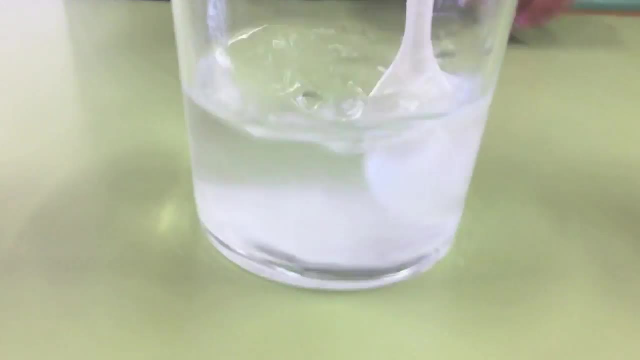 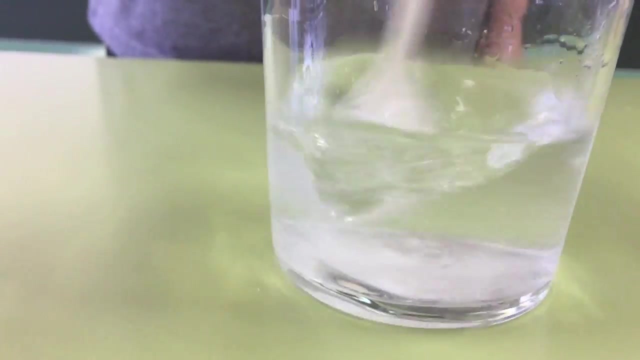 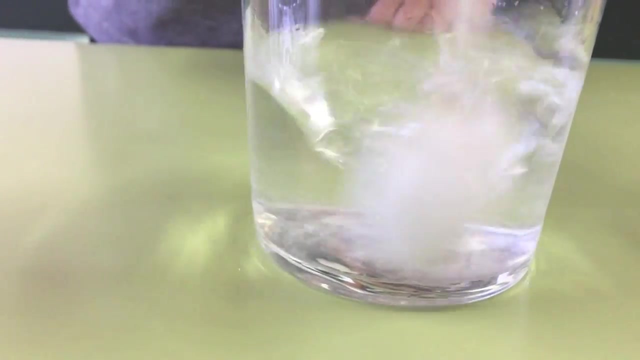 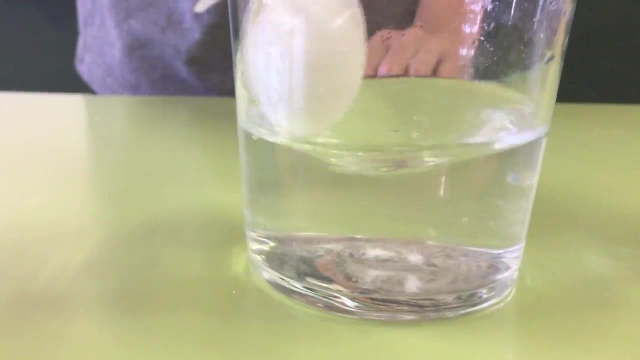 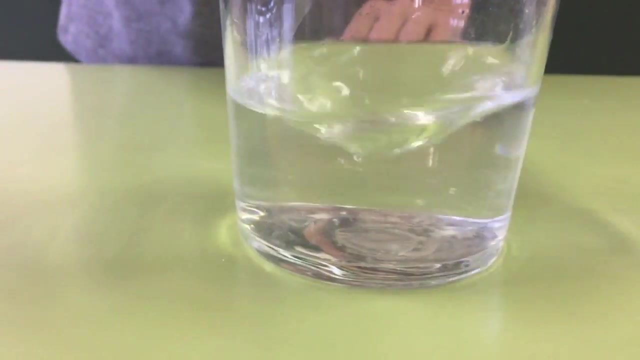 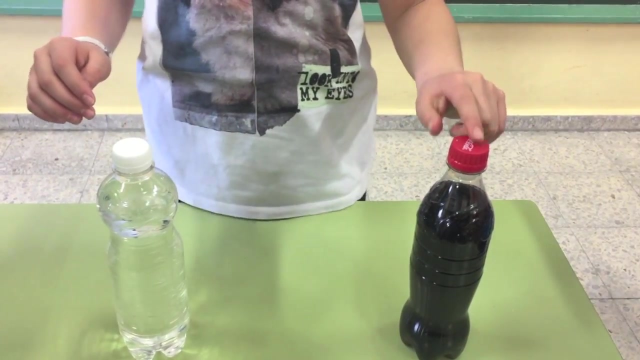 into a glass container and add some sugar or salt. In this case I add sugar. Mix it with a spoon. When the time passes, the mixture becomes a homogeneous solution, because you cannot see the components. This is another example of solution: Here we have coke and here soda. 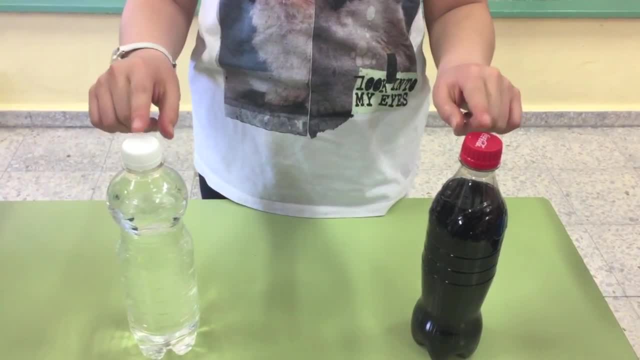 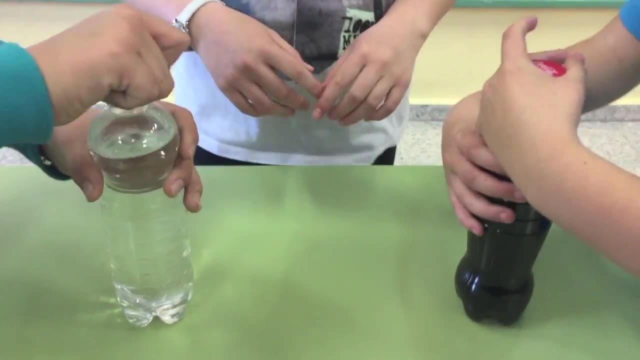 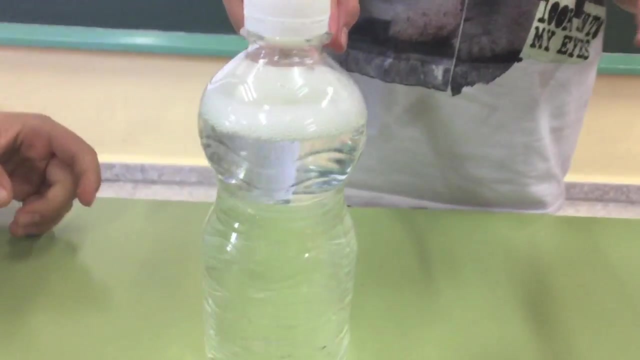 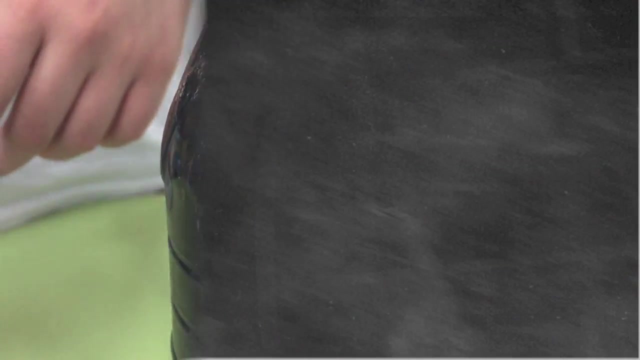 Now we don't see the components, but if we open the coke and the soda we can see the bubbles of carbon dioxide. Here are the bubbles: Eat, See money. Know Eat science. 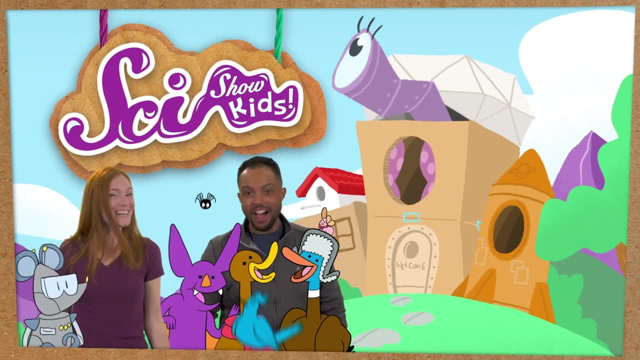 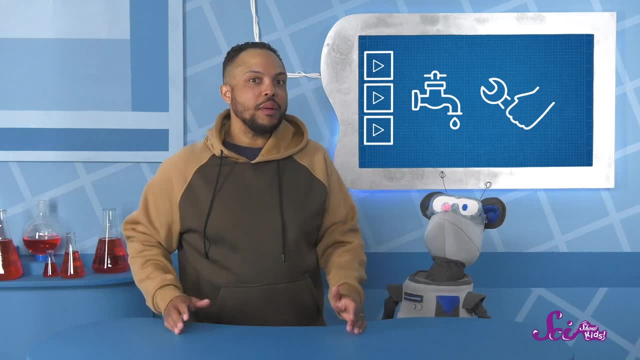 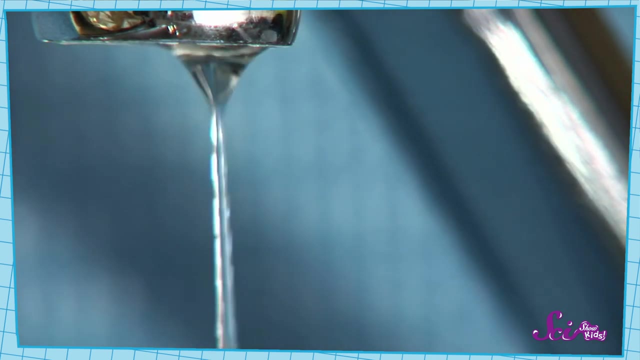 Oh, hey, there. I was just looking up information on how to fix a faucet. I turned off the kitchen faucet after washing my hands and noticed that there was still some water dripping out of it, And I don't want to waste water. Oh, don't worry, Squeaks. 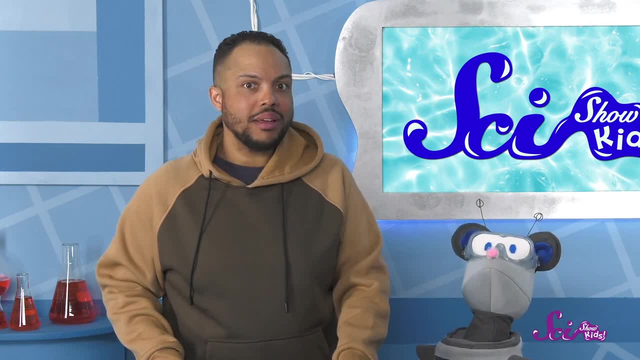 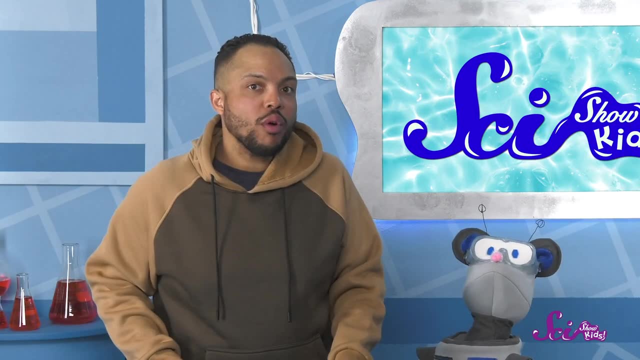 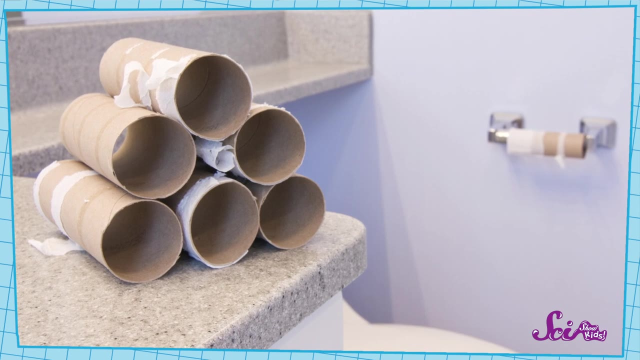 Squeaks is worried that if we waste too much water the world could completely run out, And I can see why you would think that Sometimes when we waste something or use more than we need, we run out of it. Like if you use way too much toilet paper in the bathroom, soon you won't have any. 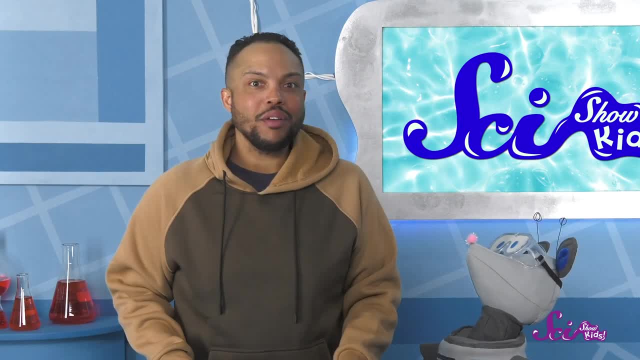 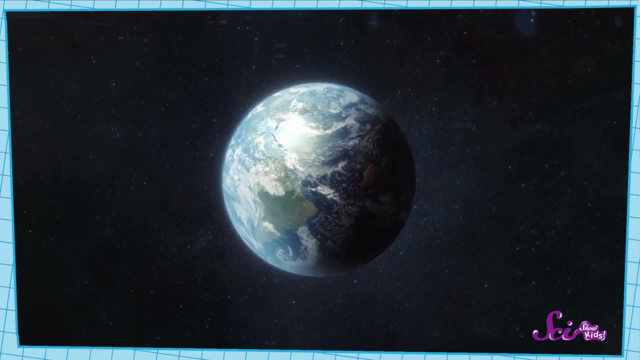 left, But I'm happy to say that the Earth isn't going to completely run out of water. Our planet has a lot of water. Look Squeaks. This is what the Earth looks like from outer space. All of that blue we see is ocean. 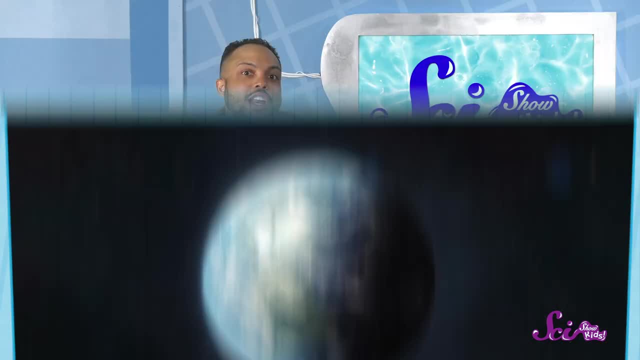 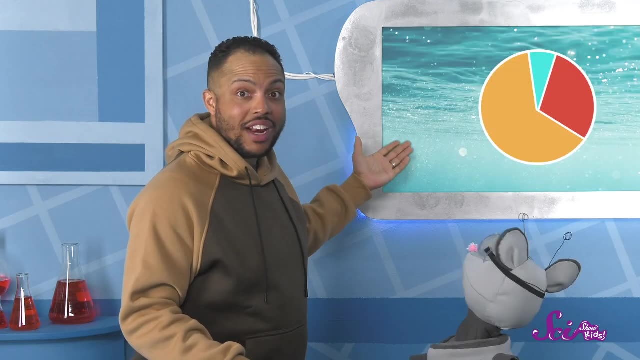 You can see that most of the Earth is covered with ocean, And oceans are full of water. In fact, they contain almost all of the water on Earth. We can show that on this chart. If this circle showed all of Earth's water, this much of it would be in the oceans. 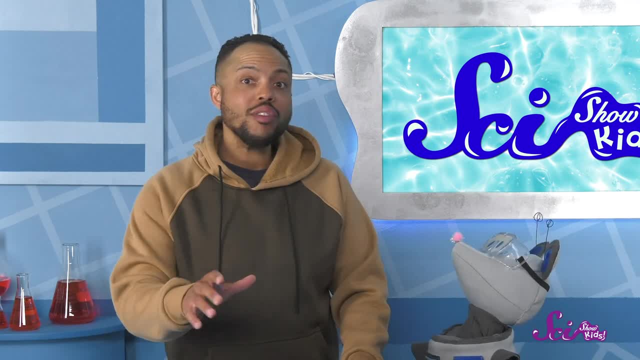 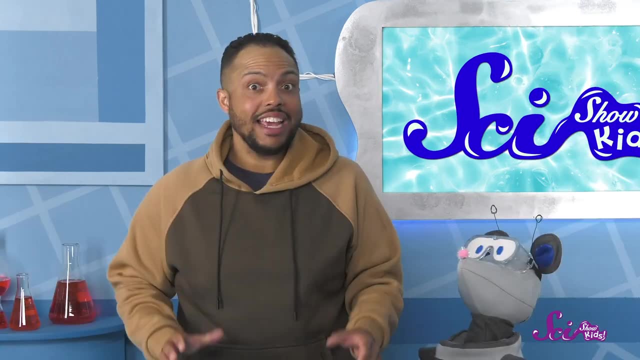 Oh, I see what you mean, Squeaks. Squeaks mentioned that even though there's lots of water in the oceans, it isn't water we can drink, And he's right. That's because ocean water is salt water. That means, well, it's got a lot of salt in it. 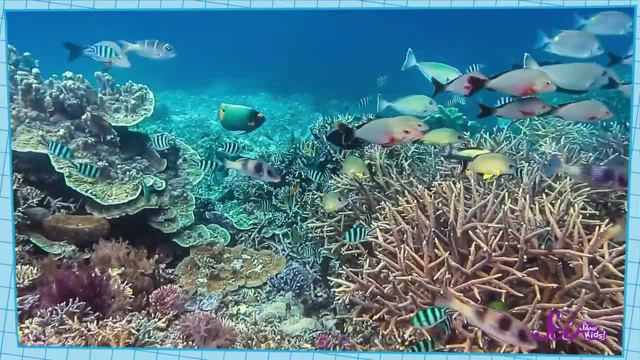 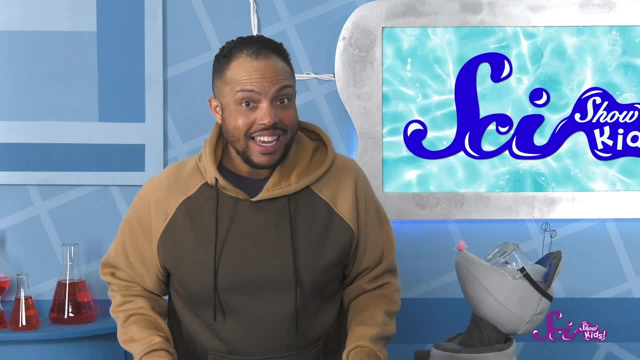 That's right And that's just fine for the animals and plants that live in the ocean. Those animals can drink salt water and the plants can use it to grow, But many of the plants and animals that live on land can't use salt water.